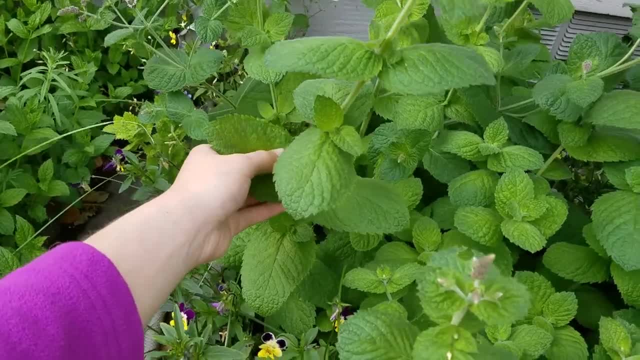 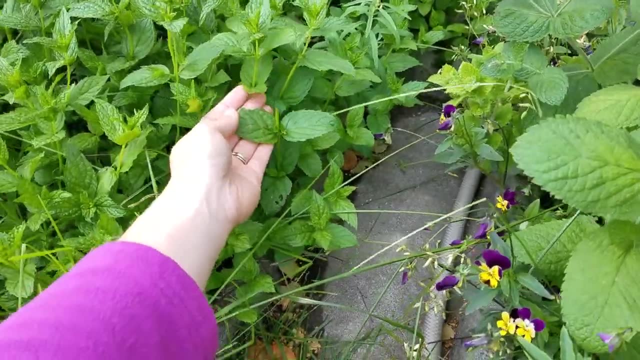 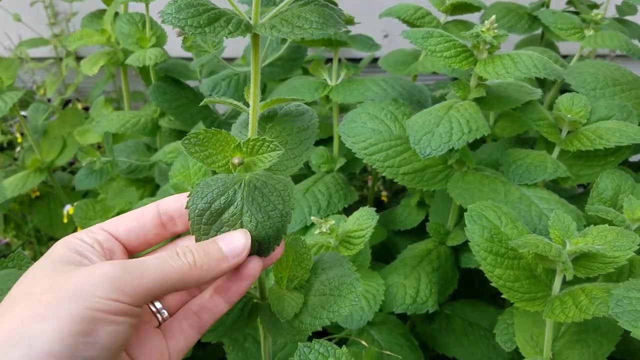 apple mint and I'll show you one of these leaves. You can see the size of this thing. That is a big leaf compared to some of the spearmint leaves. Apple mint, in comparison, is soft. The leaves are very soft. They're actually a little bit fuzzy and I'll try to get close on one of these. 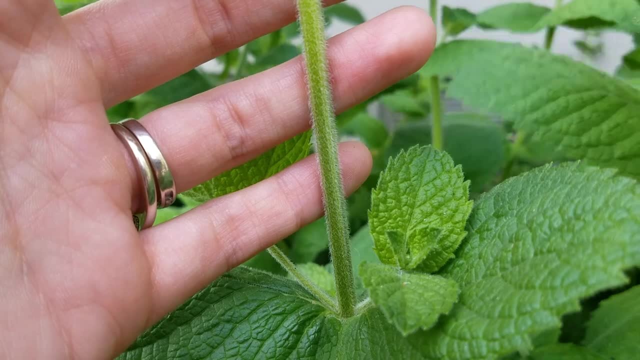 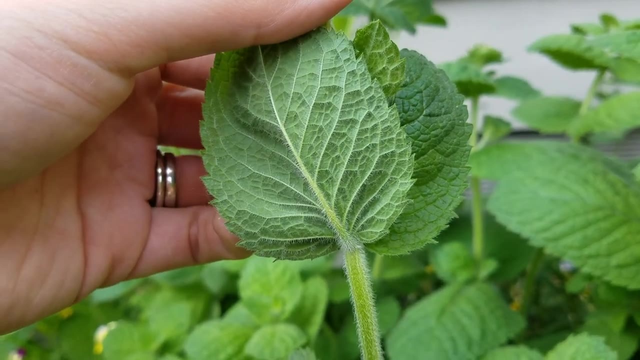 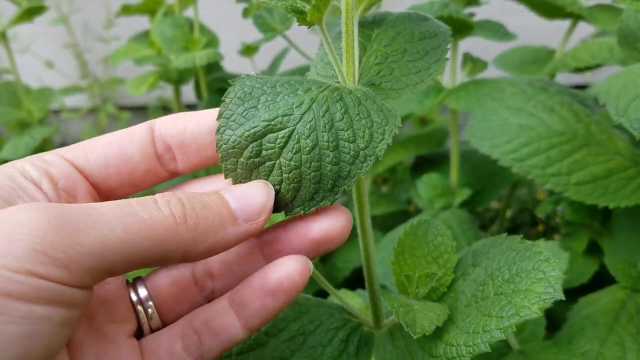 seeds. You can see what I mean. So you can see that and it's also pretty visual. on the underside of the leaves You've got all these little fuzzes and when you put it in your mouth and chew it, the fuzz isn't really. it's not a turn off, Like some plants that have those little hairs, like that can be. 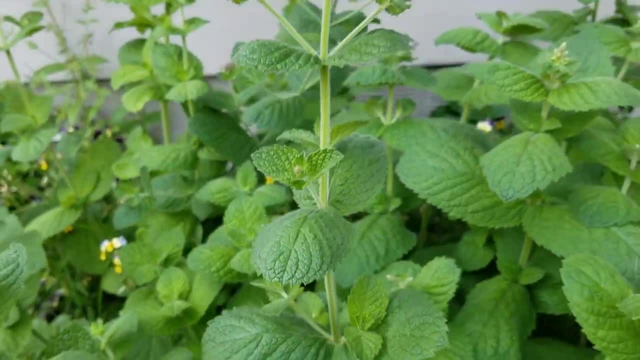 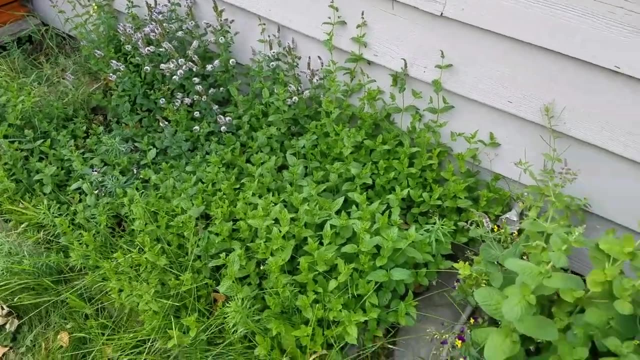 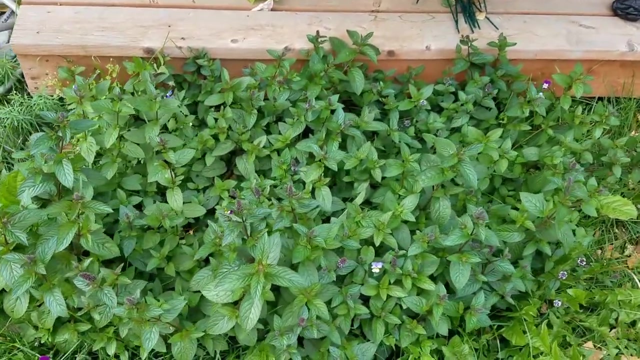 annoying to eat. It's really not that bad. The spearmint flavor, I would say The apple mint is a bit more green and planty, Whereas the apple mint is a bit sweeter. And then the third kind of mint I'll show you is called a chocolate mint. 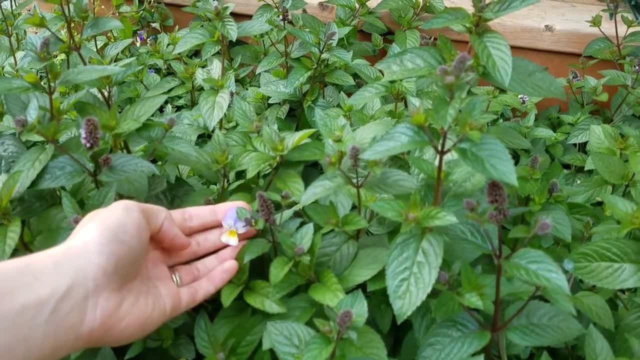 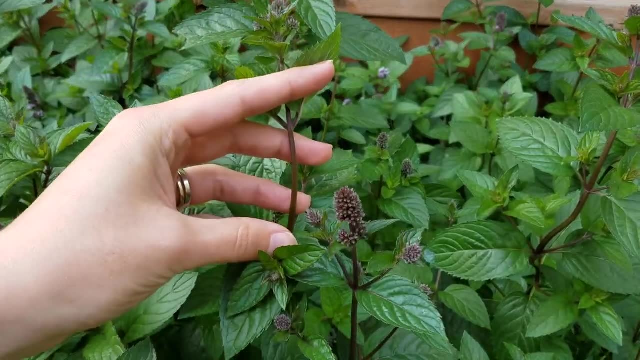 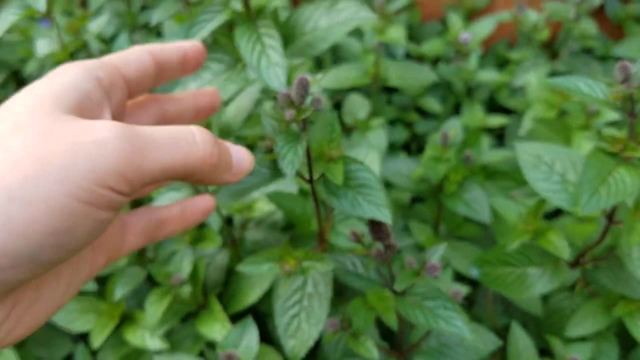 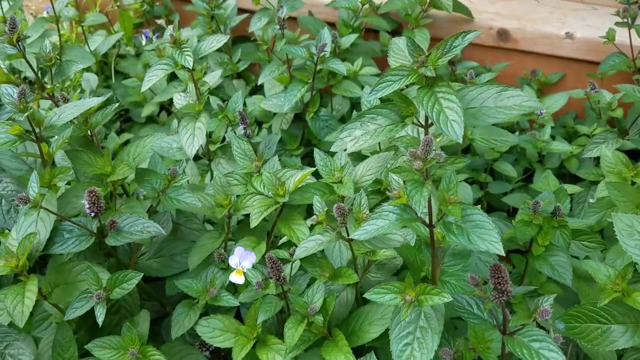 Just to ignore these little occasional volunteer wild pansies. So the chocolate mint. if you look at the stalks, the stalks are actually a purple color, And so are the veins of these leaves. Now, just on its own, you probably couldn't smell the really subtle cocoa scent to it. 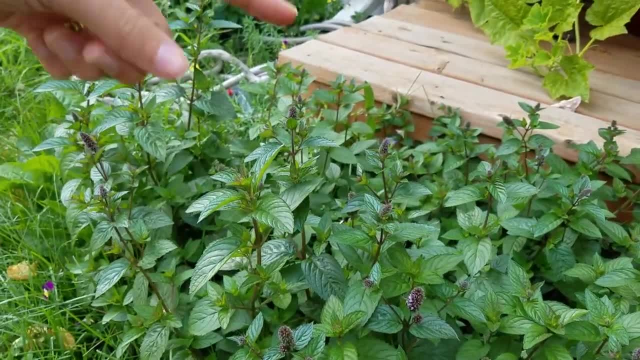 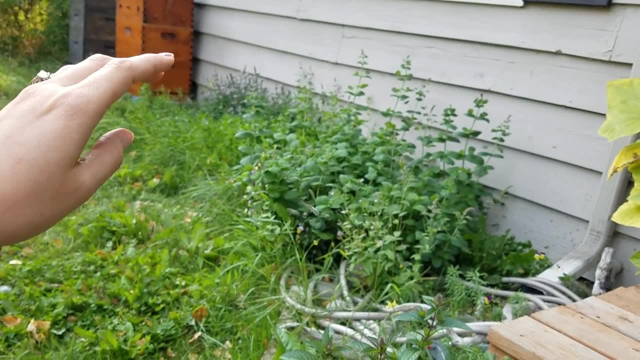 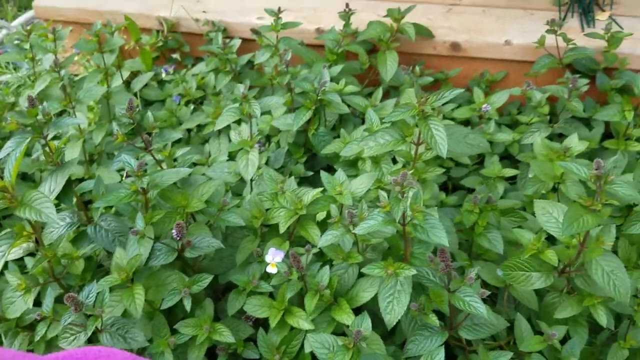 But if you're smelling a chocolate mint, right this patch, and then you smell an apple mint and then you smell a spearmint, then you can definitely smell and taste the differences between these mints. I would say that the spearmint definitely holds up the best in the wind compared to the other mints. 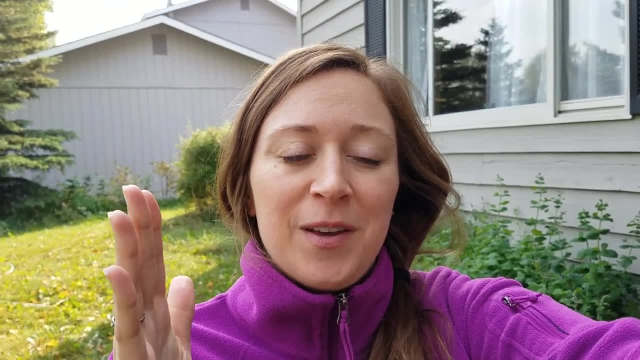 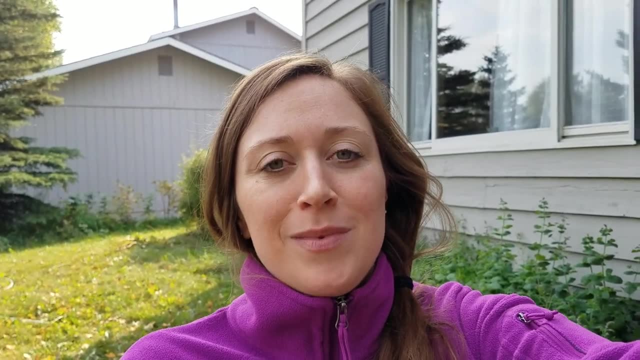 The apple mint. it's just getting so tall it's having a hard time. Every time it's windy, or whenever I go to water it, all the little stems get knocked over and then they pop back up the next day. So I'd say if you live in a very windy area, spearmint might be the best for you.